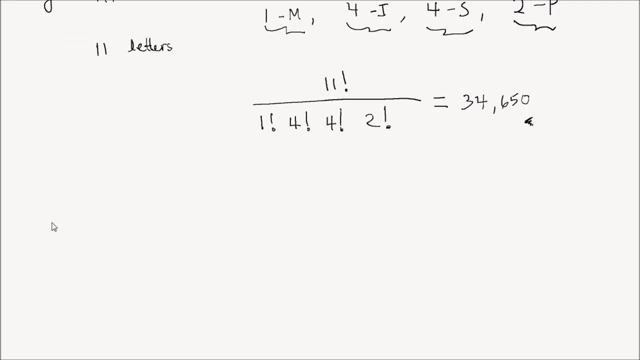 In the first part of lecture number 4, we looked at permutation And we said a permutation of k objects from n objects is an ordered sequence of k objects selected from a pool of n without replacement. But in this lecture we're going to look at combinations instead of permutations. 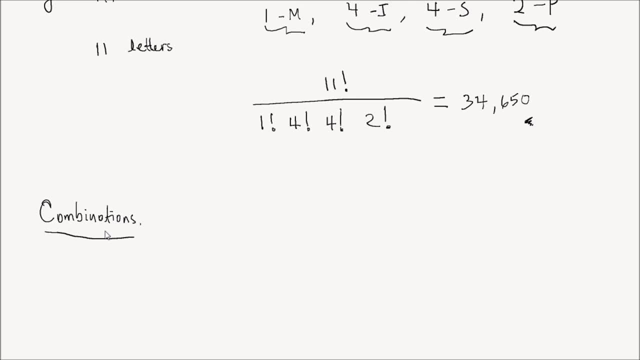 And again I'm going to use an example to illustrate what we mean by combinations. A simple example. Let's say we have 4 students and we would like to send 2 of them, or we would like to select 2 of them, to attend a conference. 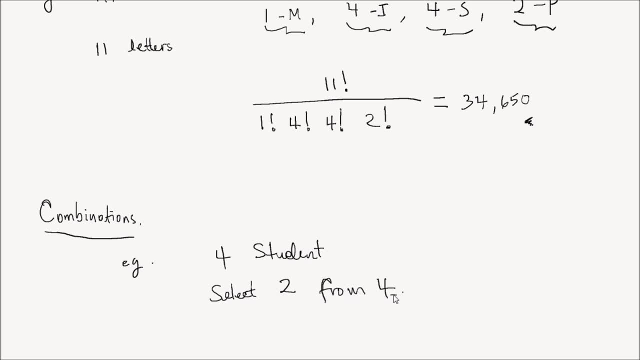 So select 2 from 4.. For simplicity, let's say we have person A, person B, person C and person D, So I could select A and B to attend the conference. Or I could select person A and person C to attend the conference. 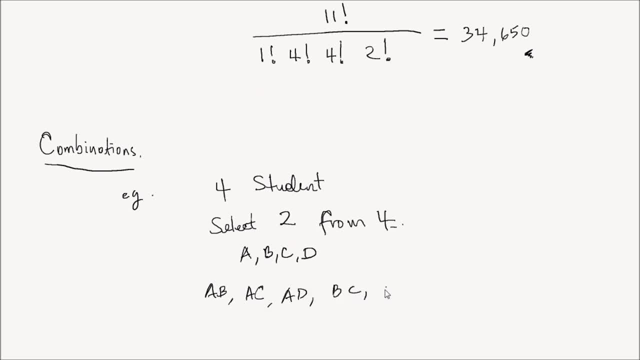 A and D, B and C, C and D and what else? B and D. So I have 6 possible ways Of selecting 2 students from 4 students. What you notice here is that selecting A first followed by B is the same as selecting B first followed by A. 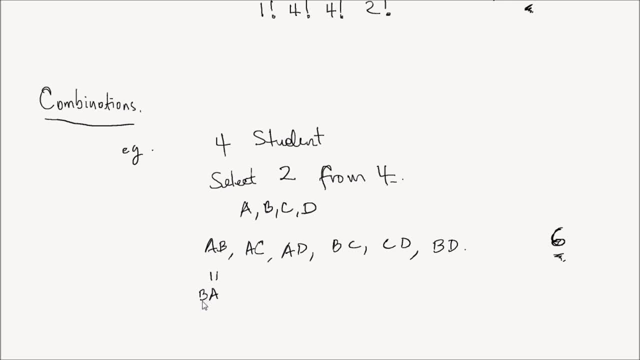 This was not the case for permutations And permutations we had person A coming in first, followed by person B coming in second. is a different ordering from person B coming in first and person A coming in second, But in combinations order does not matter. 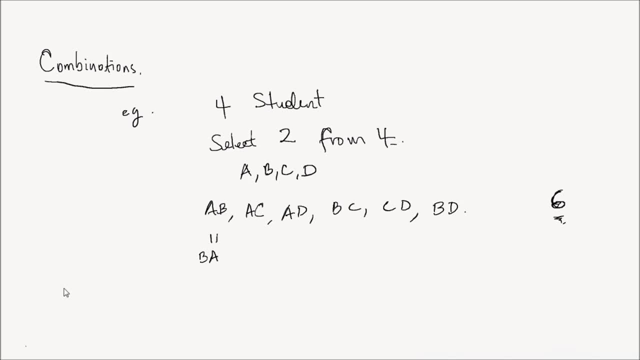 And the notation we use for combinations is N choose K. This is if we would like to select K objects from a pool of N objects without regard to order, as N choose K, And the notation which is often used actually is N C, K. 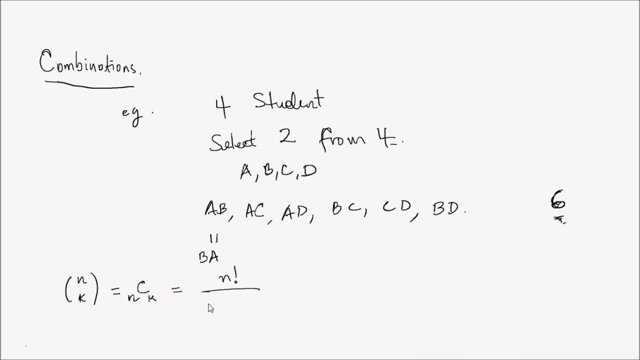 which is given by N factorial divided by K factorial times: N minus K factorial. Let me extend this example that I gave you first. Now, instead of 4 students, maybe I have 24 students in the classroom and of which I would like to select 6 to attend a conference. 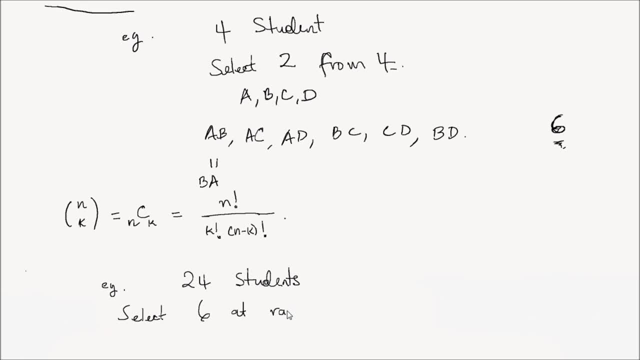 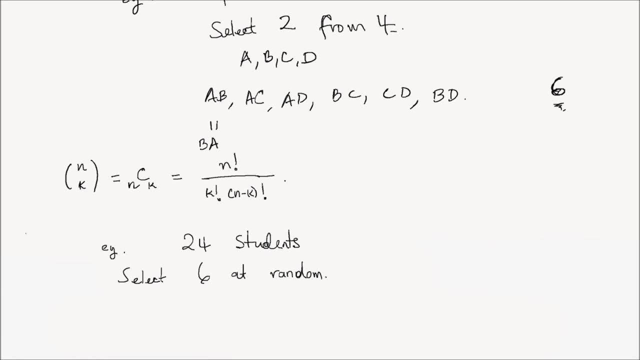 Select 6 at random to attend a conference, And how many ways can I choose 6 students from 24 students? I can find that by calculating 24, choose 6.. If you like this notation, you can use it: 24 C, 6.. 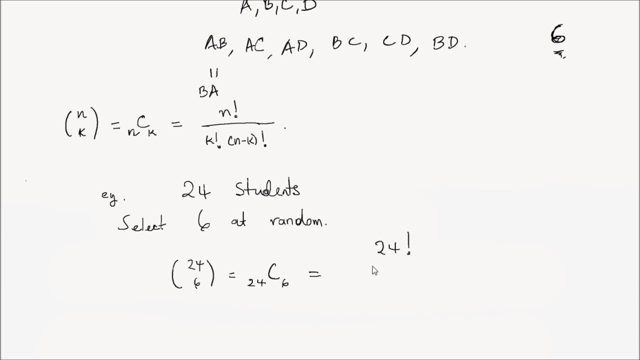 And that is equal to 24 factorial divided by 6 factorial times 24 minus 6 factorial. 24 minus 6 is 18.. 24 factorial divided by 6 factorial times 18 factorial is equal to 134,596.. 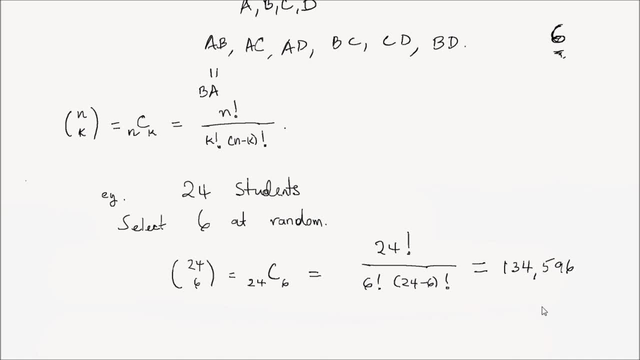 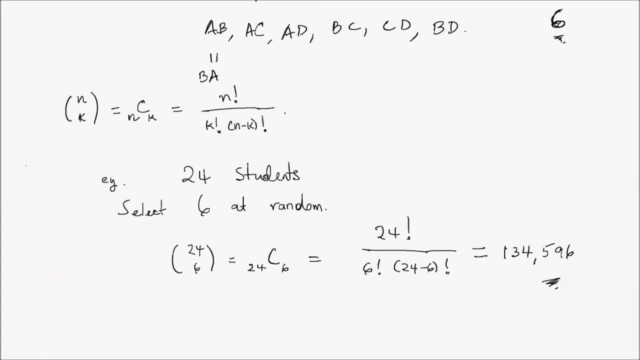 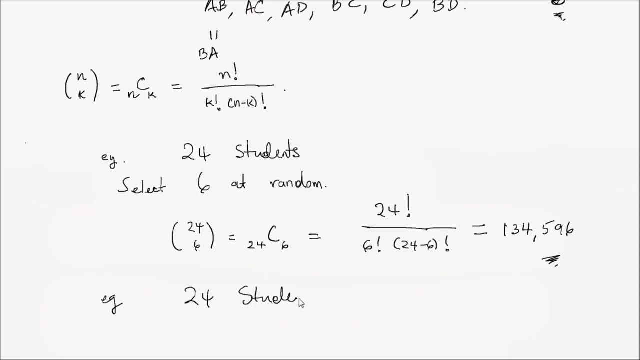 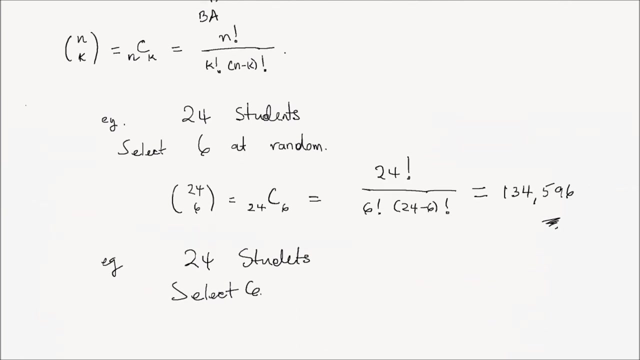 134,596 possible ways of selecting 6 students at random from 24 students. Again, let's say I have 24 students, I still want to select 6 to attend a conference. But now I am given more information. Of the 24 students, let's say 10 of them are engineering students. 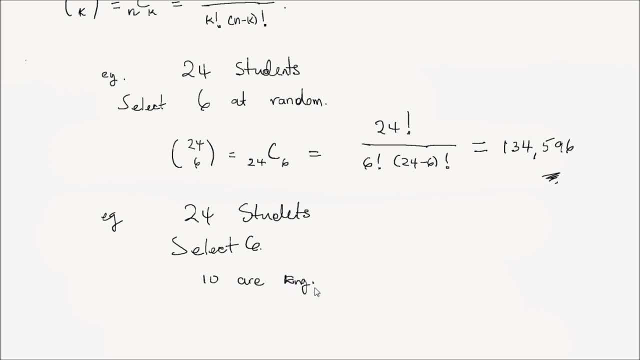 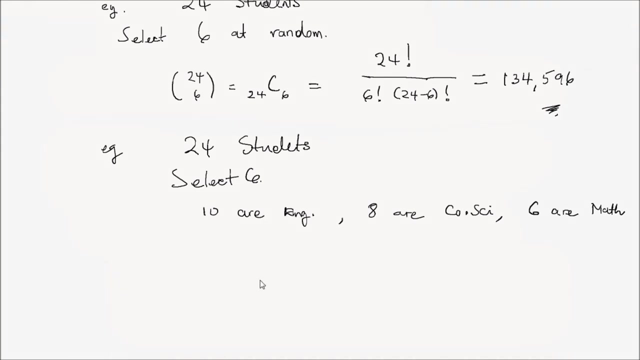 Each of them are maybe computer science students And the rest- that would be 6, are math students. Now the question is: in how many ways can I select 6 students? In the following way: I want to make sure I have 2 students from engineering, 2 students from computer science and 2 students from math. 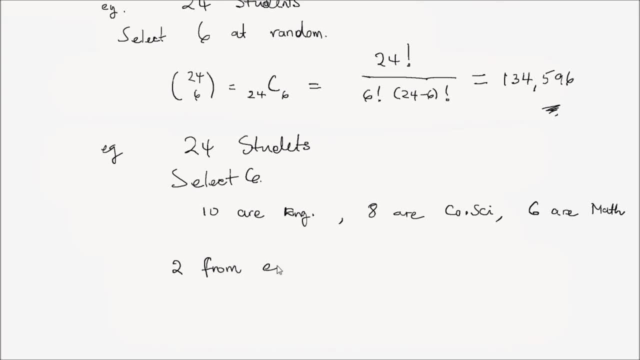 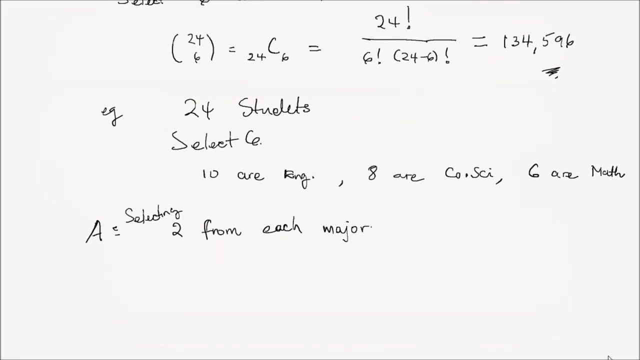 That is 2 from each major, And how many ways can I do that? Let's define event A to be the event of selecting 2 from each major. So the number of ways this event can happen, the number of ways I could select 2 students from each major and combined I could have 6 in total- is the following: 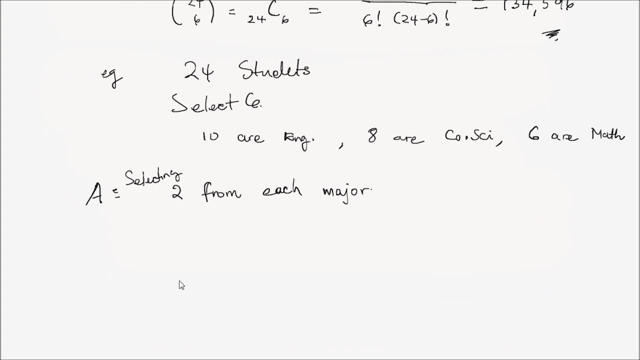 You can think of this as An experiment which is done in stages or in sequences. In the first stage, stage 1,, you select 2 from engineering students, that's from 10.. In the second stage, you select 2 from computer science students, that is, 2 from 8.. 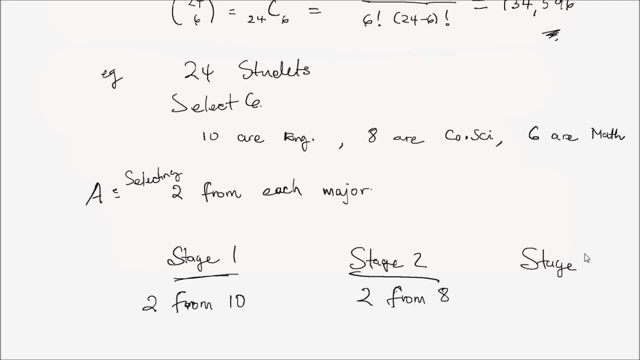 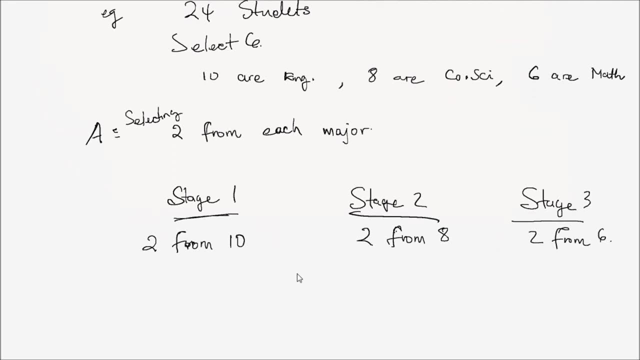 And in the third stage you select 2 from math, That's 2 from 6.. The number of ways of choosing 2 students from 10 engineering students is: 10- choose 2.. The number of ways of choosing 2 from 8 is 8- choose 2.. 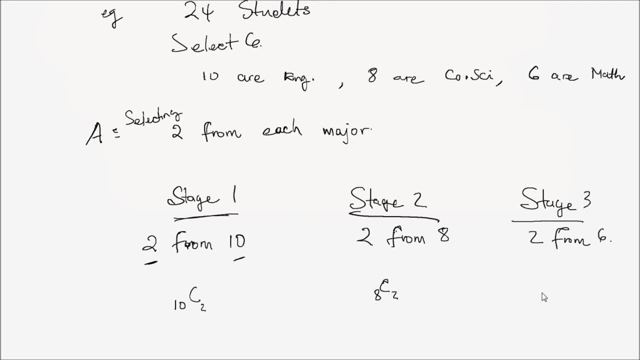 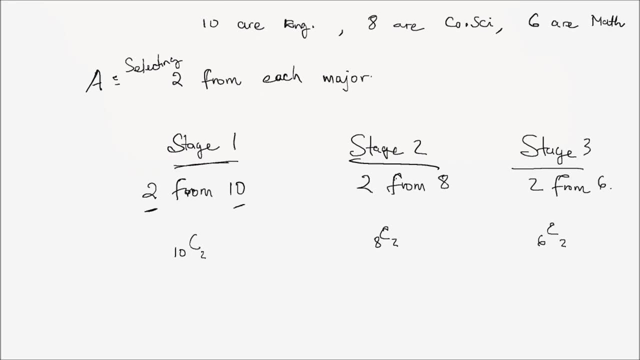 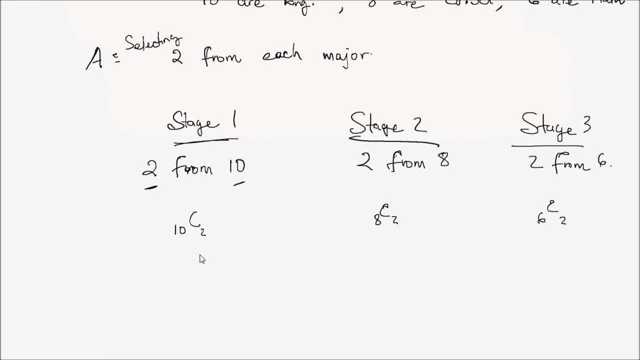 And the number of ways of choosing 2 from 6 is 6 choose 2.. By multiplication rule of counting, if I have an experiment done in sequences and each sequence has a given number of ways that it could be done, then the number of ways that event could happen, the number of ways that A could happen, 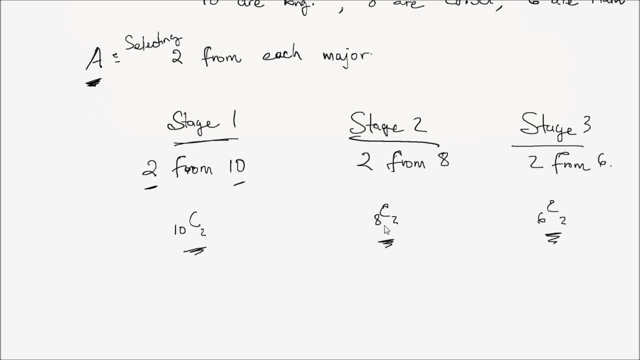 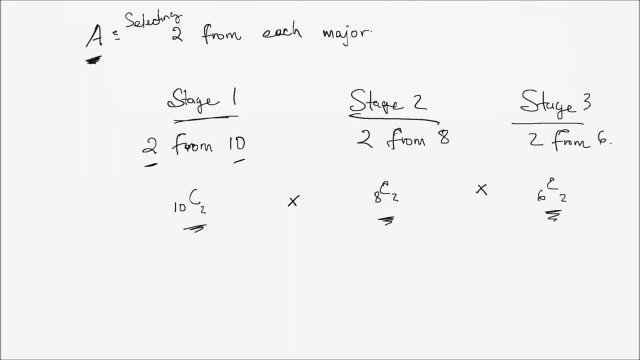 is 10, choose 2. multiplied by 8, choose 2. multiplied by 6, choose 2.. But I could also ask you: what is the probability of what was event? A Probability of selecting 2 students from each major? What is probability of A?